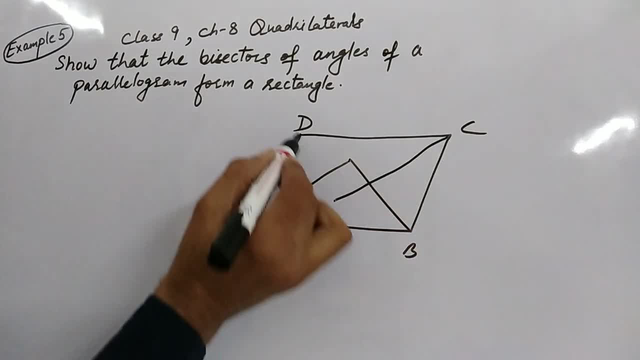 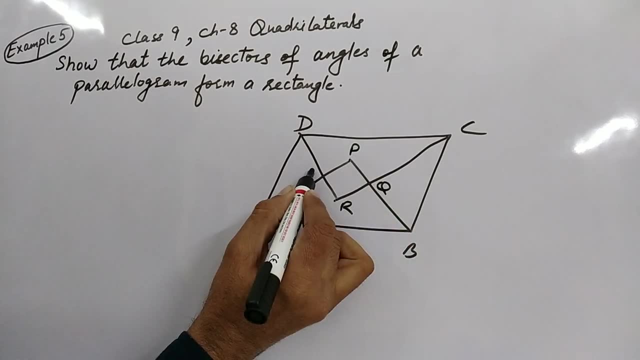 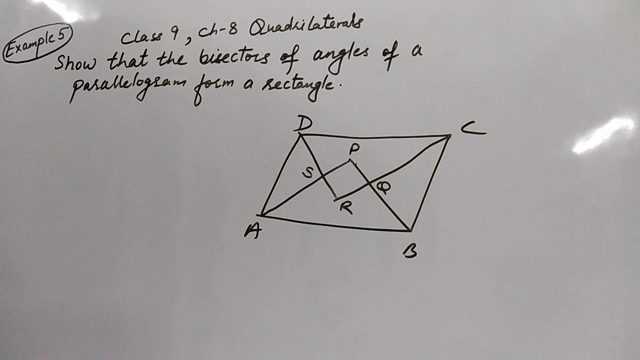 angle B, this is bisector of angle C and this is bisector of angle D. So suppose this is PQRS. So this PQRS we need to prove as a rectangle. So we need to prove PQRS as a rectangle. and ABCD. 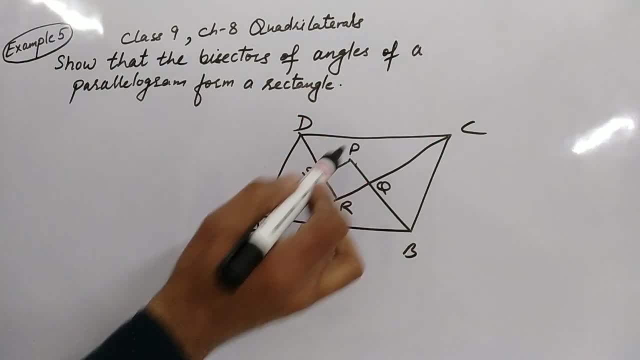 is parallelogram given to us. So AP is the bisector of angle A, BP is bisector of angle B, CR is bisector of angle C and DR is bisector of angle D. So let's do What we do, we will make. 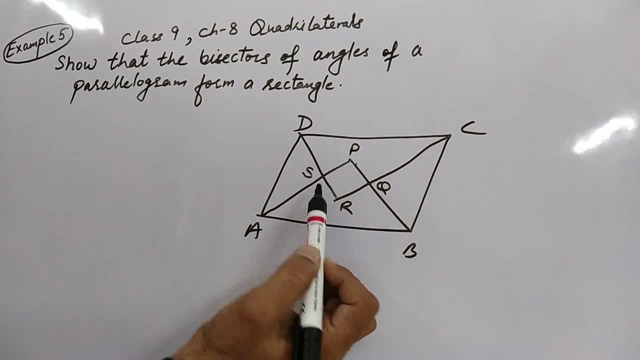 each angle 90 degree and we can say that if each angle of this quadrilateral PQRS as a 90 degree, so it is a rectangle. So our motive is to make each one of these angles in quadrilateral PQRS as 90 degree, So we can say: this is a rectangle. So our way is this. So let's start. 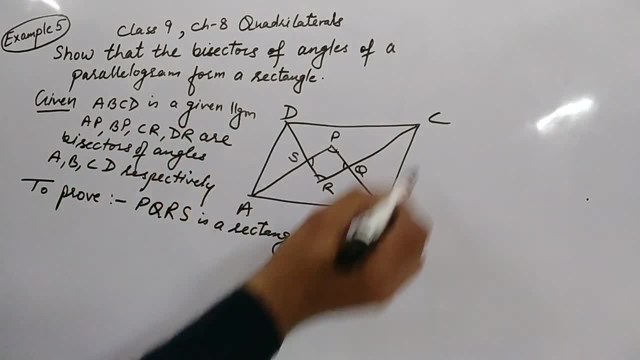 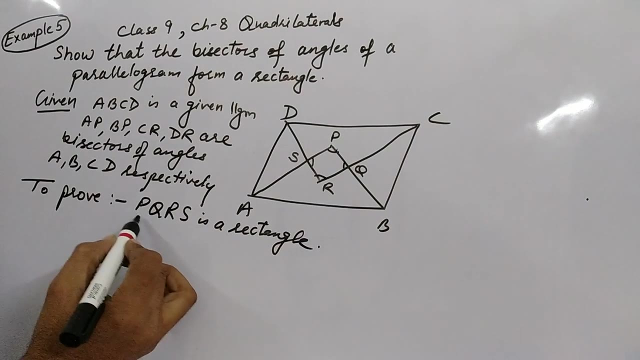 So this is written. ABCD is a given parallelogram. AP, BP, CR and DR are the bisectors of angle A, angle B, angle C and angle D respectively. And to prove this is: PQRS is a rectangle. So let's do this proof. 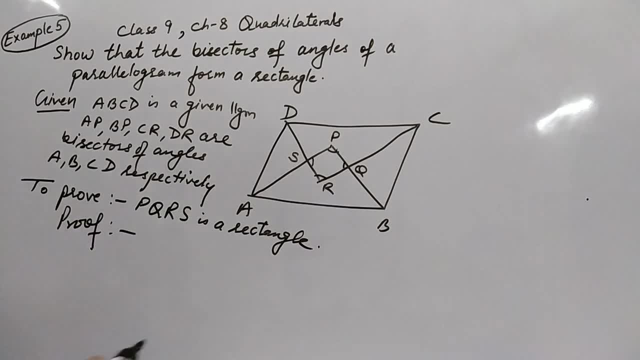 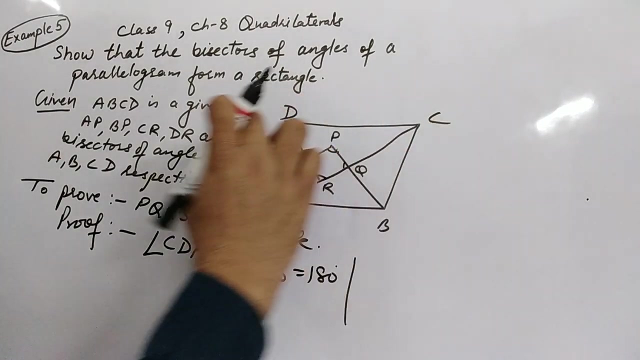 Proof. So what we do? angle D, this full angle D, you can write angle CDA. This is CDA angle Plus angle DAB. This angle is 180 degree because these are consecutive interior angles, because these two lines are parallel. CD is parallel to AB, AD is transversal. So this angle D plus this, 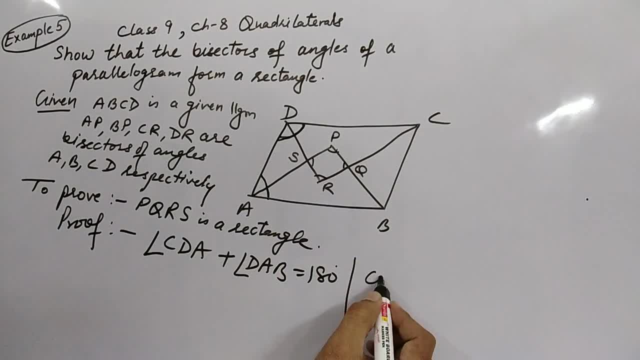 angle BA is equal to 180 degree. So we write here: reason: co-interior angles. We call these as co-interior angles, So then take half on both sides So it becomes half of angle CDA plus half of angle DAB is half of 180.. 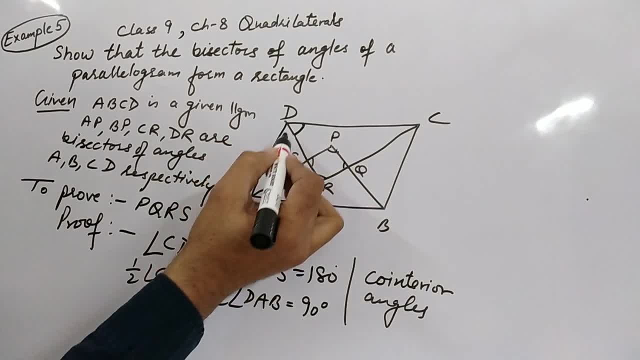 That is a 90 degree. So half of angle CDA. Suppose this is angle 1 and this is angle 2.. So half of angle CDA is angle 1 because DR is bisector of angle D. So half of angle. 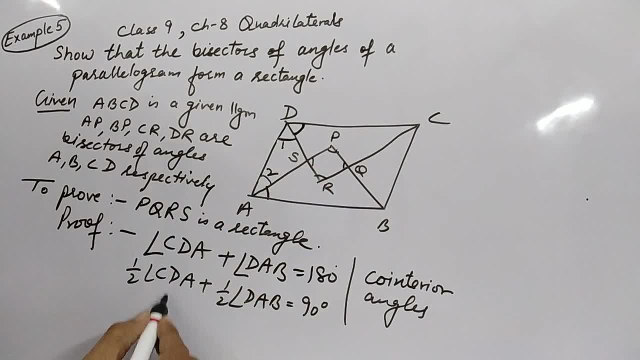 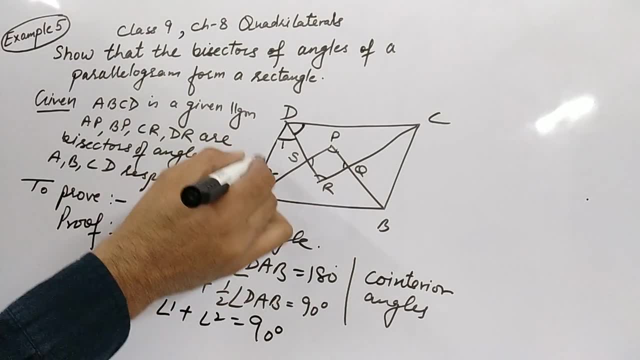 CDA will be angle 1 or either angle. this also, So I can write here in place of this. angle 1 plus half of angle DAB will be: angle 2 is 90 degree. So angle 1 plus angle 2 is 90 degree. This is. 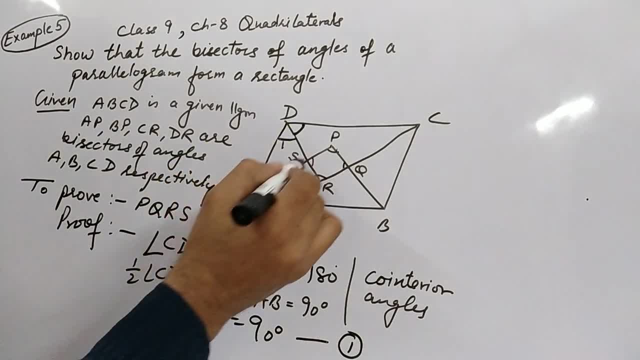 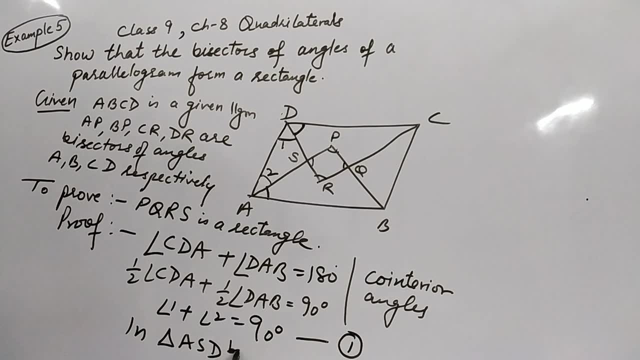 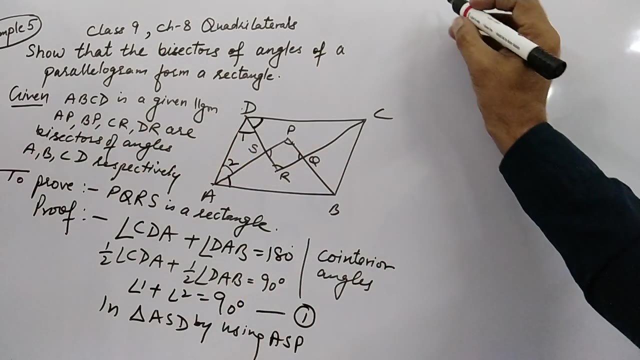 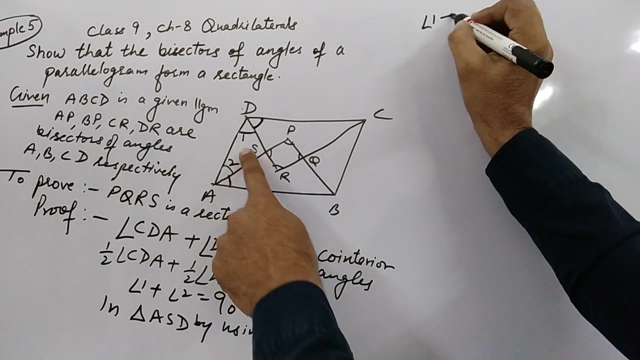 equation number 1.. So we will apply in triangle ASD angle sum property. So in triangle ASD, by using angle sum property, So it becomes angle sum property in this triangle, So it becomes angle 1 plus angle 2 plus angle this. 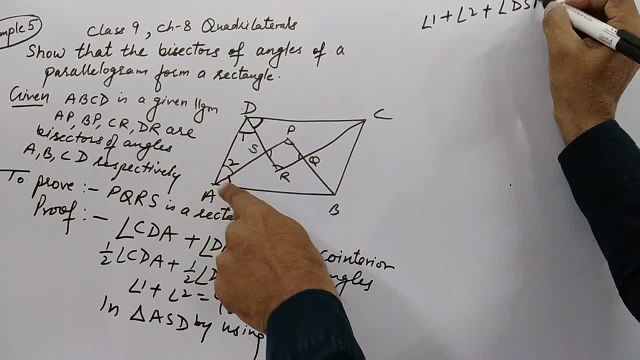 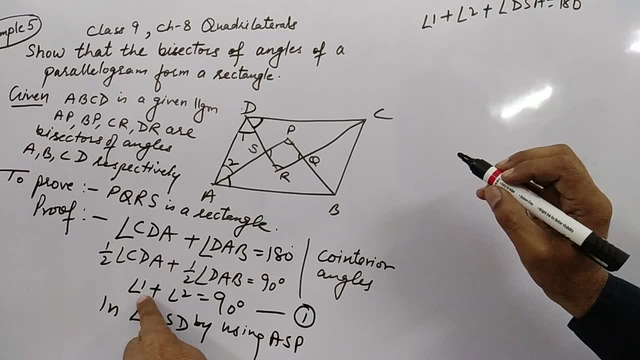 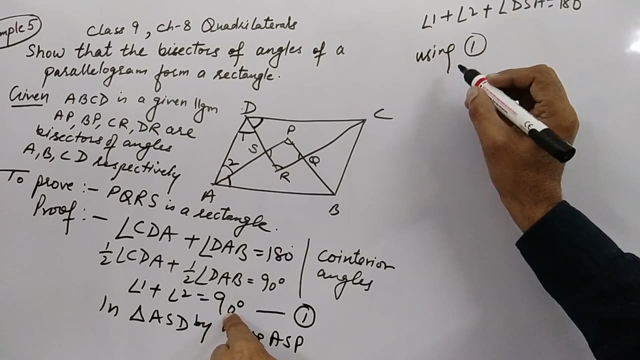 S angle. We write this as angle. DSA is 180 degree, So here from here we can use angle 1 plus 2 as 90 degree. So using 1 in place of 1 plus 2, we can write 90 degree. So write 90 degree, So we can. 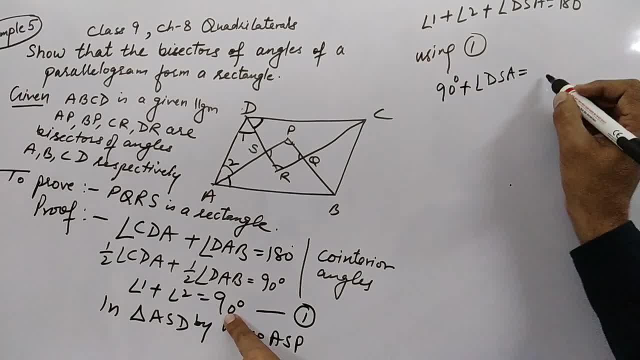 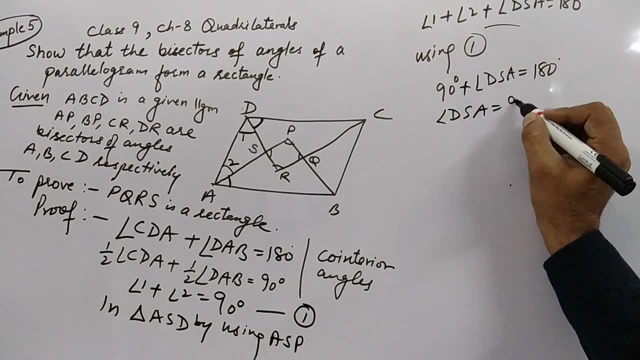 write: 90 degree plus angle DSA is 180 degree. So angle DSA will be 180 minus 90. So it becomes 90 degree. So this angle is 90 degree. Similarly, or you can say: if this angle is 90 degree, then 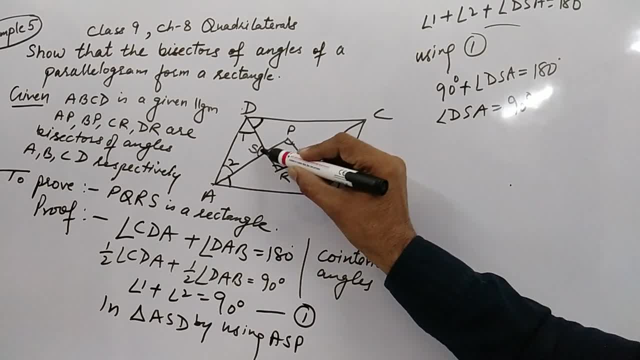 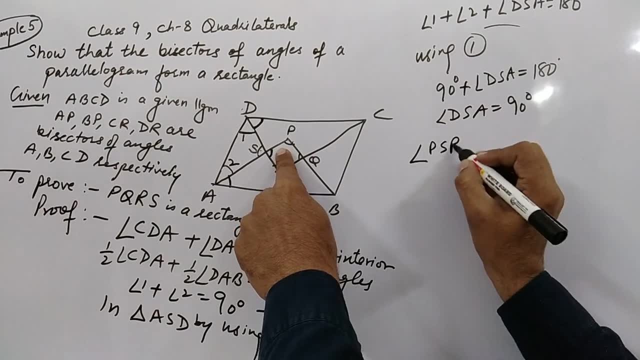 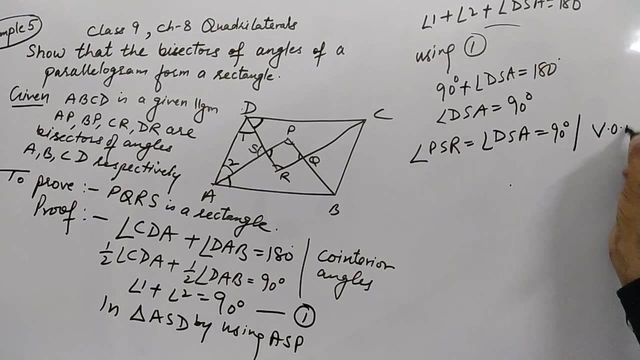 this angle will also be 90 degree, because this is: these two are vertically opposite angles. So we write here: angle PSR. This is angle PSR is equal to angle DSA, say 90 degree, because these are vertically opposite angles, So this angle is 90 degree. 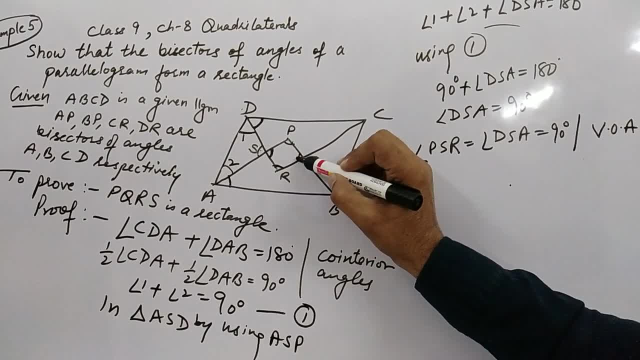 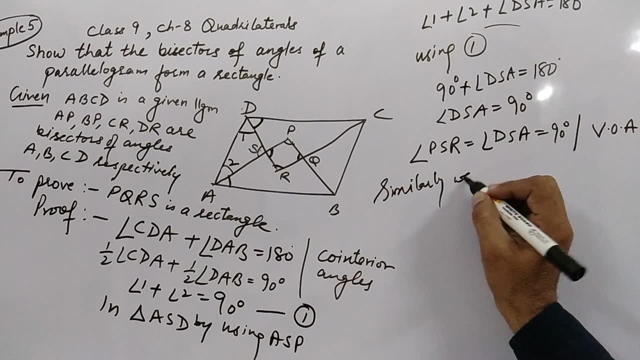 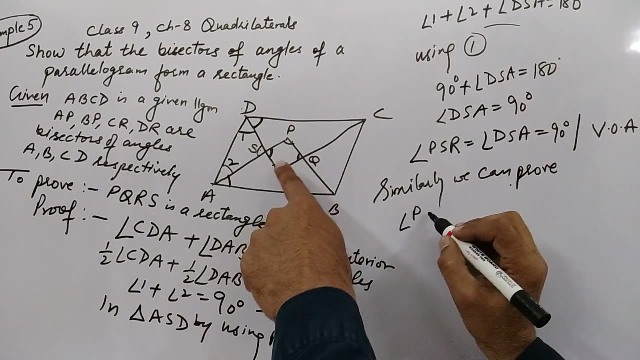 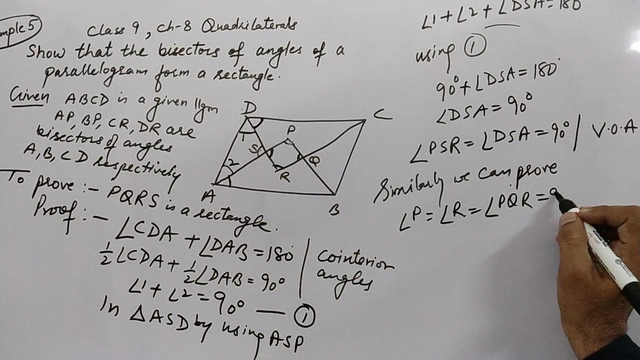 coming. Similarly we can prove: this also 90 degree, this also 90 degree, this also 90 degree. So we can write similarly. similarly we can prove. we can prove: angle P is equal to angle R, is equal to angle PQR, also 90 degree. Hence each angle of PQRS is 90 degree.